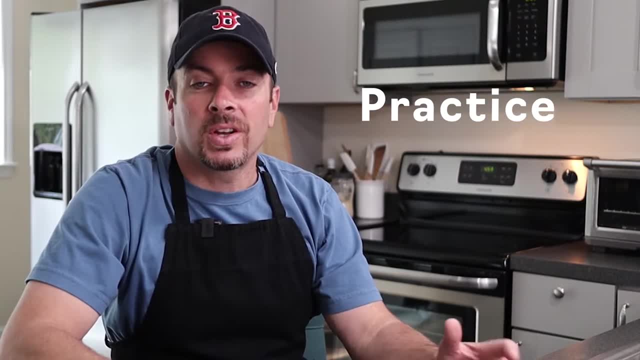 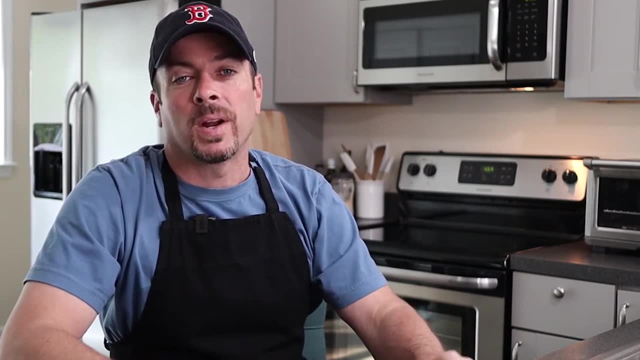 perfect is really important with cooking. The more you cook, the better you're going to get. And now when you practice something- say, your practice can golf or baseball or one of those- you're also going to mess up. So that's something to really 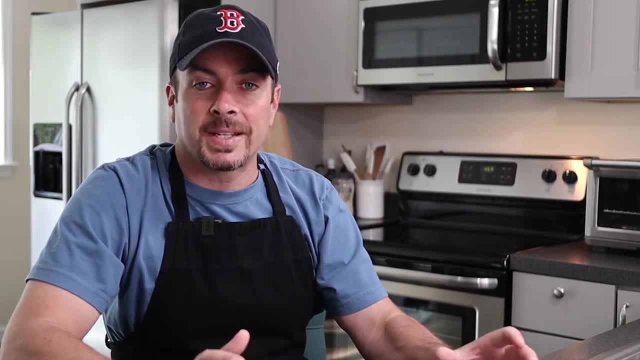 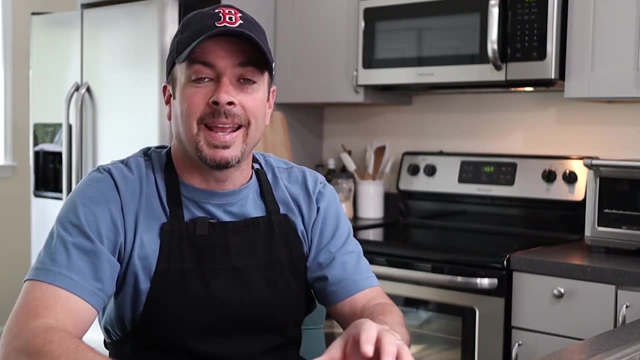 think about You're not going to be perfect. A lot of people when they do recipes, they're following something step by step and they're worried about messing it up. But the beauty about practice cooking and doing it over and over, you're going to get better at it. 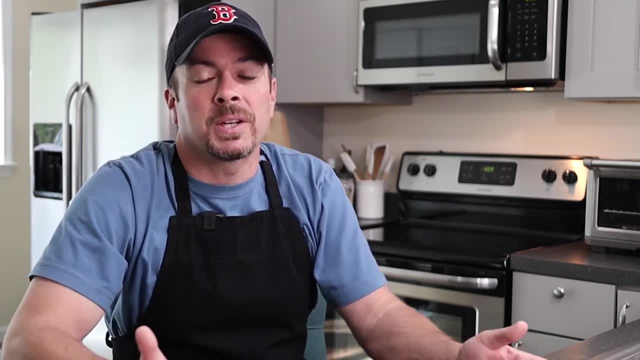 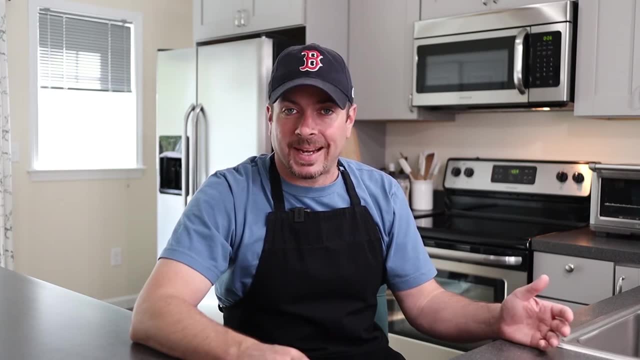 You're going to fail. You're going to mess up. We all do, especially as home cooks. We're not professional chefs, We're just cooks. And the thing is we all fail. Just the other night I was making soup and I asked my wife to watch it, And then I 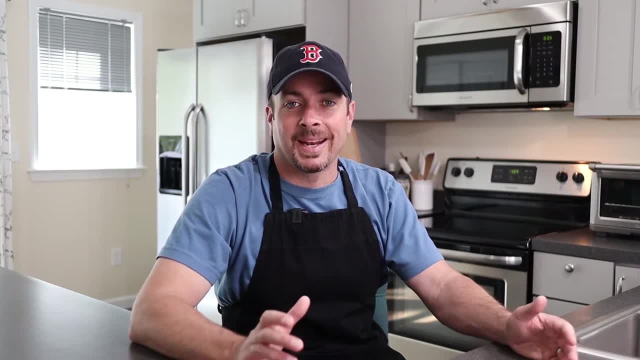 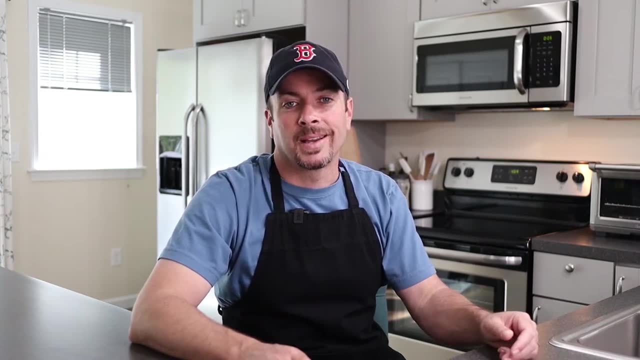 was supposed to be watching it And I was just sauteing the vegetables in the beginning and I burnt them on the bottom of the pan. We all do it, We all make mistakes, We learn from it, but we keep cooking. So the next thing I want to talk about: when you learn how to cook, especially if 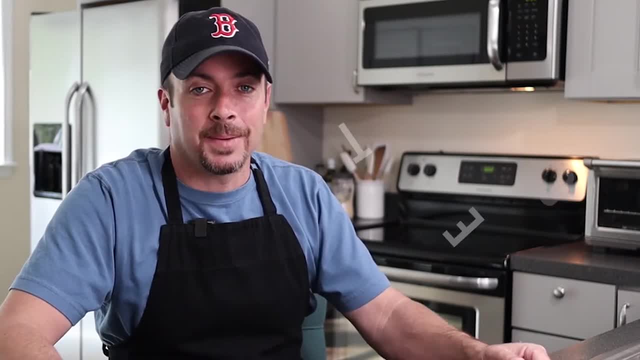 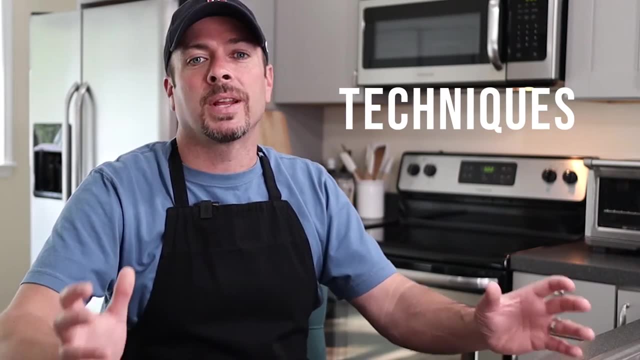 you're a beginner is learn the fundamentals of certain techniques. Now I'm talking about braising, sauteing, baking. all you know: sauteing and braising. You might sound like whoa, that sounds a little complex, but it really isn't, And it's really. 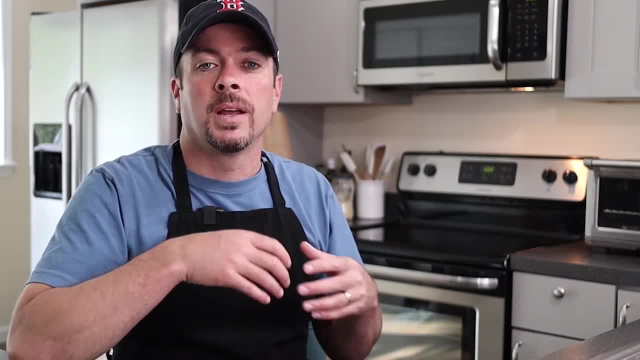 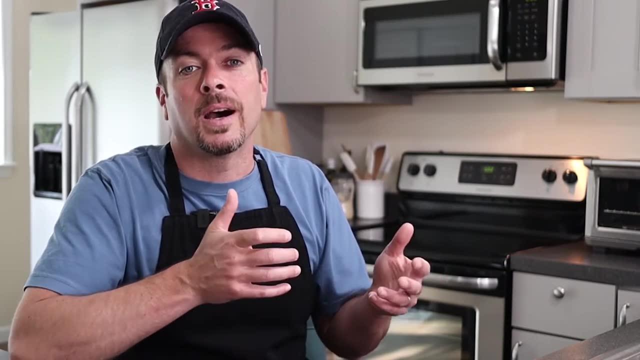 simple. A lot of them. you know the cooking that people do day to day as a home cook usually incorporate these types of cooking, but they might not exactly know what they are. So take braising, for example. you're taking a cut of meat, whether it's chicken or beef. sometimes it's a tougher cut. 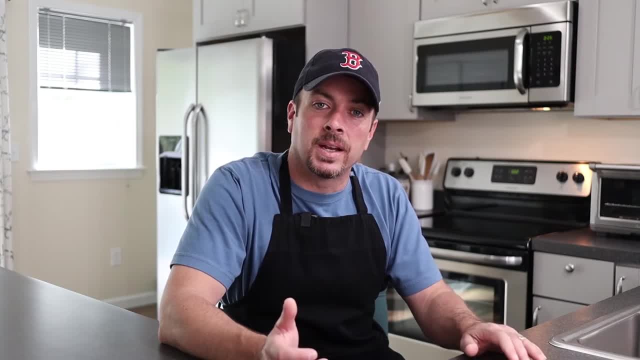 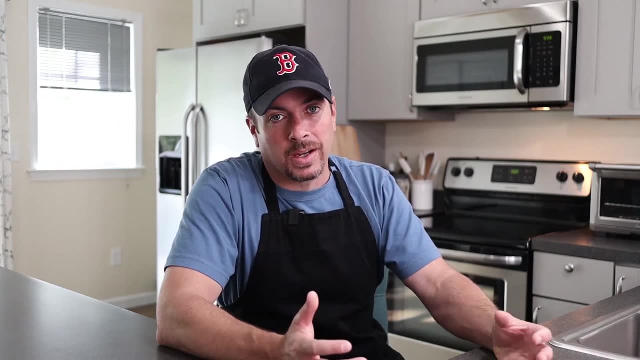 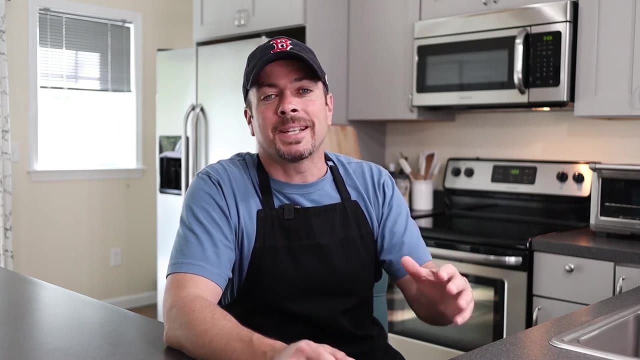 of meat and you're just cooking it in a little bit of liquid over time And that liquid is going to help the time and the slower the cook and the lower temperature is going to help that connective tissue break apart a little more and make the meat even more tender. And it's that simple, You're. 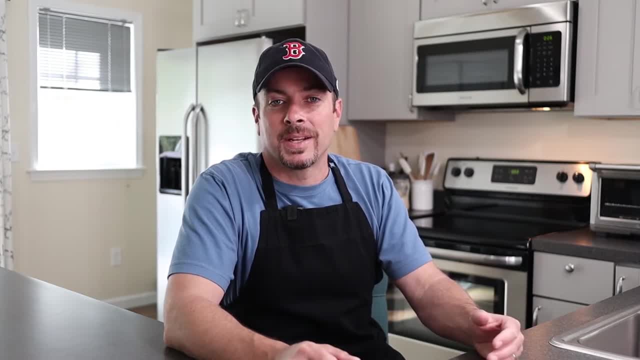 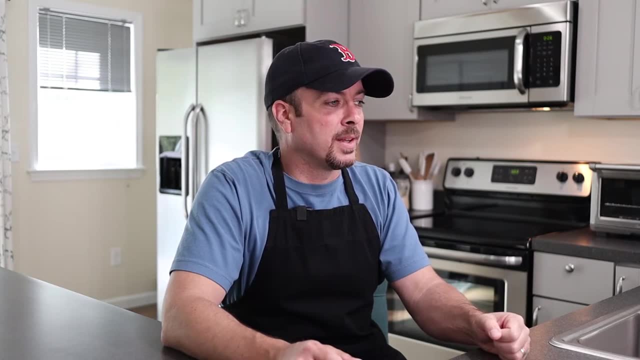 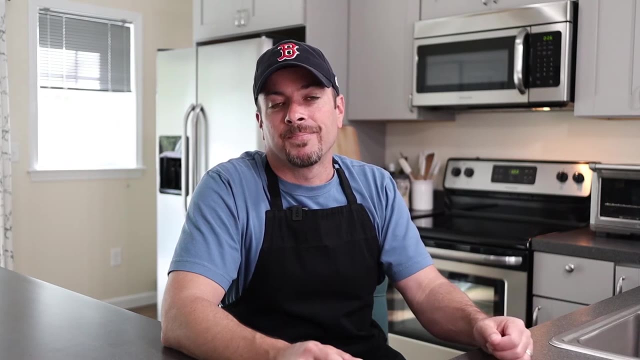 cooking the meat in a little bit of liquid, whether this braising liquid is a chicken stock or you used, you know. you deglaze your pan with a wine or vinegar and then you added a little bit of water and that's what you use to braise in. It's really simple, but that's something you want to learn and 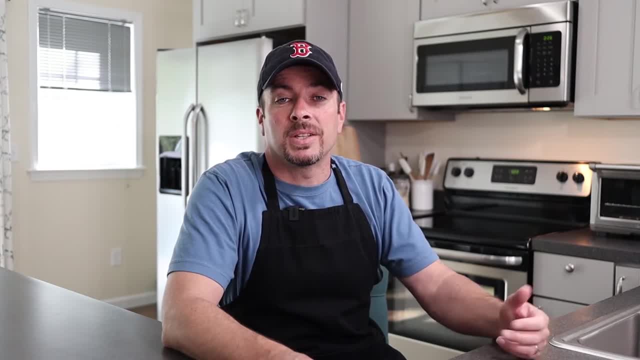 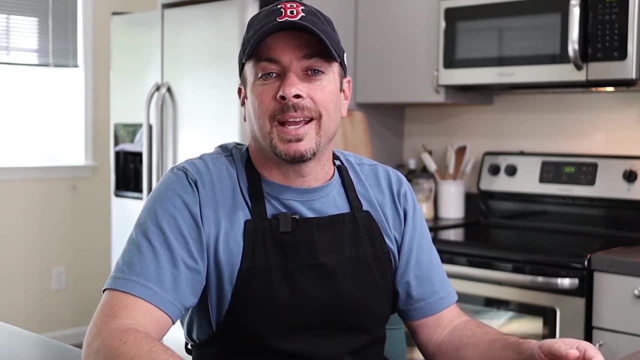 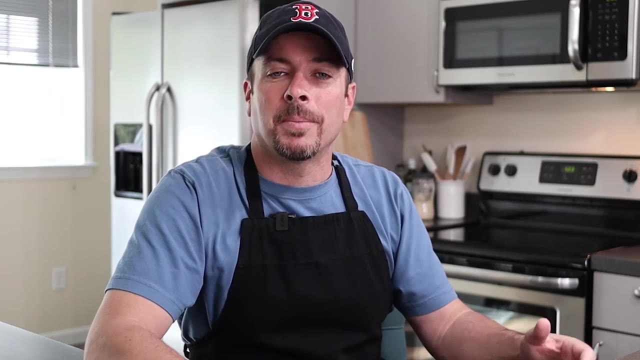 it. on my channel I have one. I did a video on braising chicken and I did one on braising beef. Another great skill you're going to learn is to saute. You want to be able to saute your vegetables, your meats, your chicken, your beef, and it's really simple. So sauteing sounds like it might. 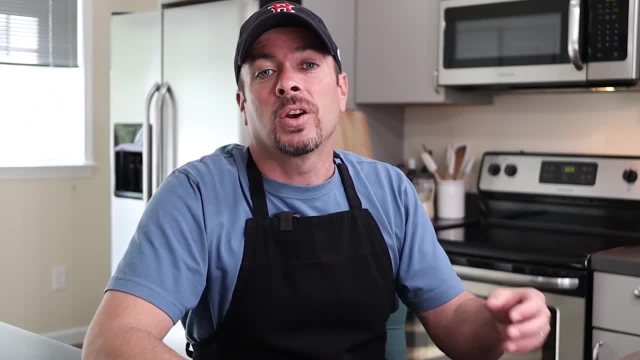 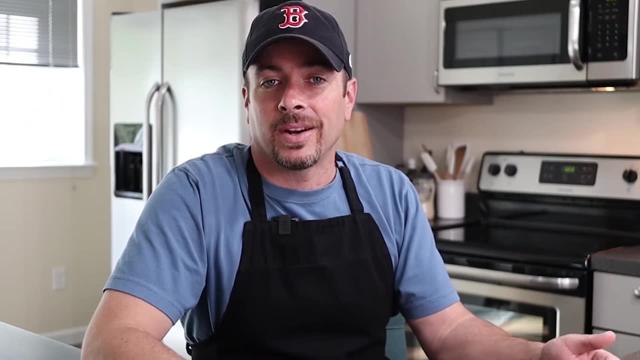 sound a little bit intimidating, but really sauteing is cooking a meat, usually a little pieces of meat and a bit of fat on a higher heat, But usually it's it's quick cooking and you're going to cook it. you're going to cook it fast And we do this with 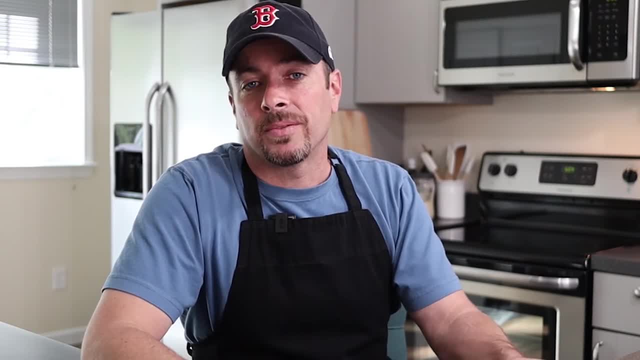 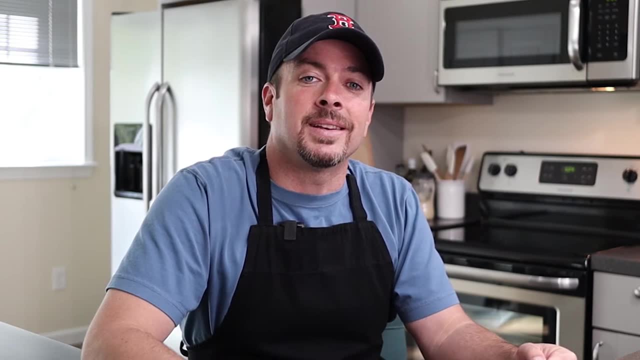 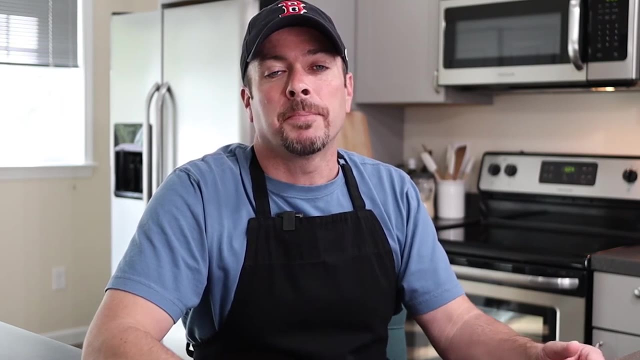 olive oils and avocado oils or chicken fat and stuff like that. But sauteing is really simple and it's a fundamental you should learn and it's really simple. And then there's always baking. So I'm not talking baking just brownies and cookies, but using your oven to bake a whole chicken. So 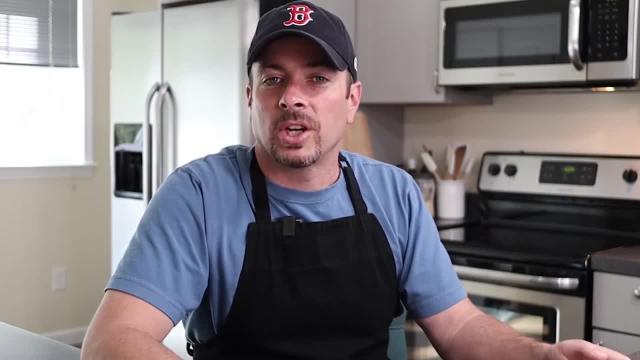 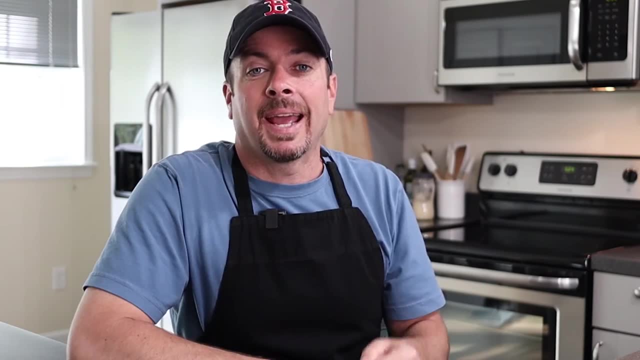 you're going to roast a whole chicken for an hour or bake pork chops. You're really using that oven as a container for heat for a certain amount of time. And now another one you want to learn if you have the availability to be able to do this- is: 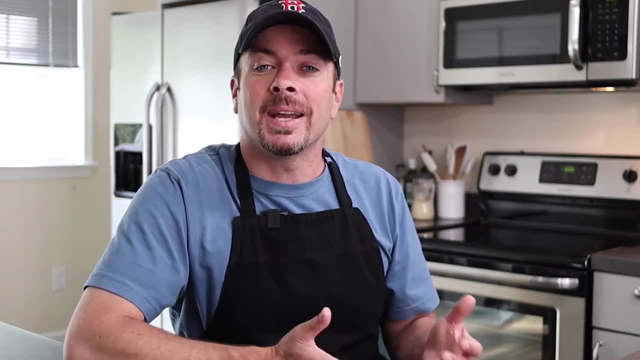 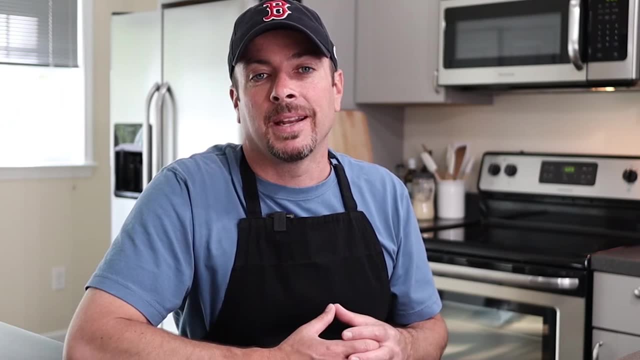 grilling- Like grilling- is really simple and it might seem intimidating, But in my videos you're going to see how you control your heat and you control your meat to be able to grill it to the temperature that you want. So we're going to cover grilling, and this is another. 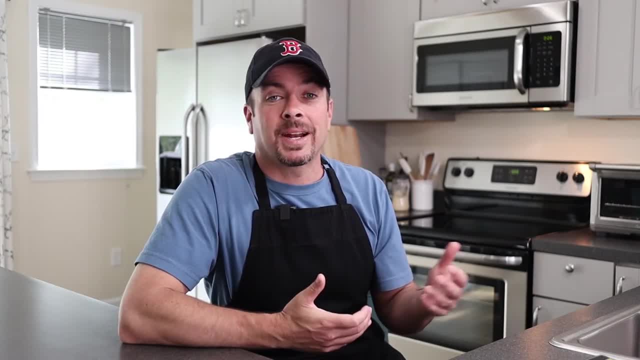 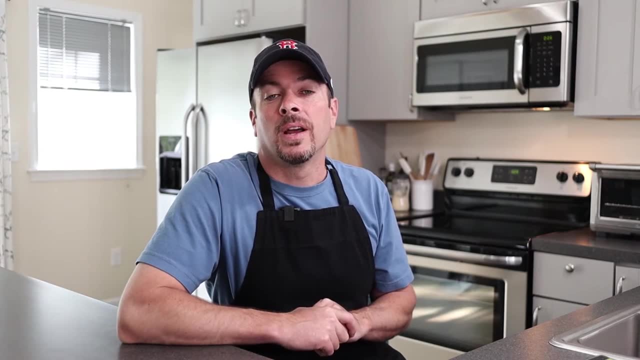 great way to learn how to cook Now with the techniques that I was telling you about. is there one that you struggle with? If there is, let me know in the comments below and maybe we can help you with a video that I could do on that specific topic or the technique that you're having a hard time with. But let me know. 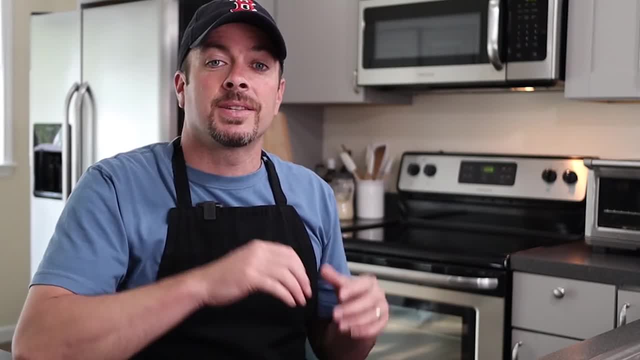 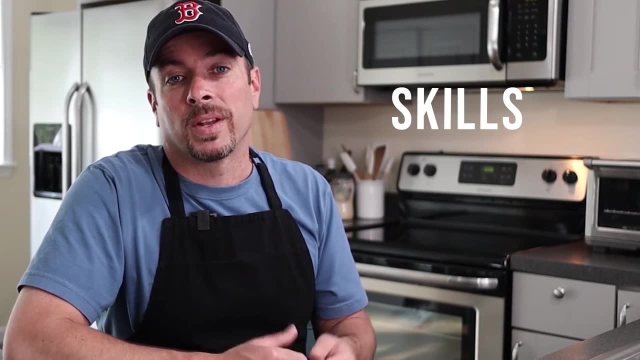 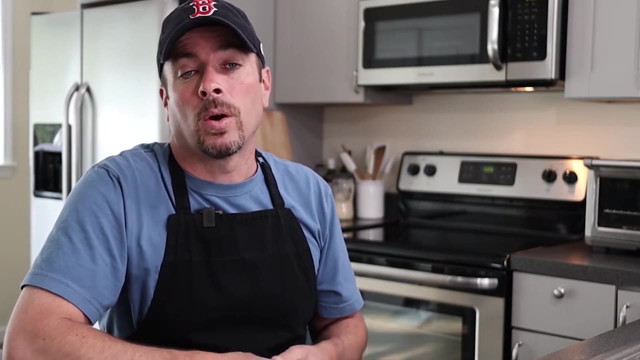 in the comments. Another thing you want to learn as a beginner is specific skills, like your knife skills: Cutting different types of vegetables and getting comfortable with a chef knife, a paring knife, understanding the differences between what you would use: a chef knife or a paring knife or possibly a boning knife. I got a great 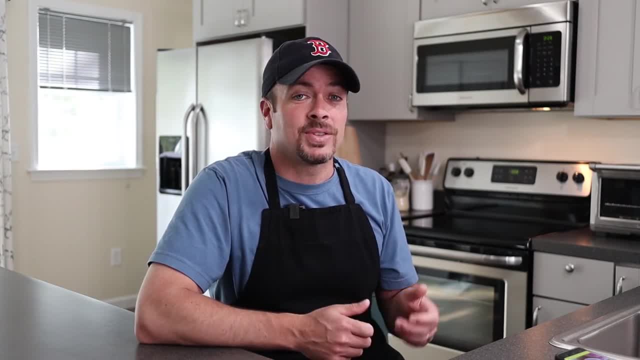 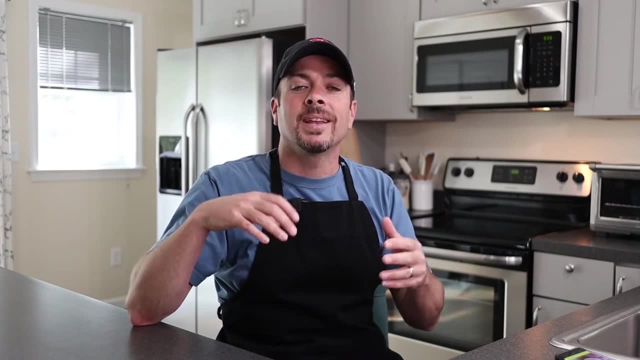 video that I just did, that I took apart a whole chicken and I used a boning knife. And you might only take apart a whole chicken. You're like Bob, that sounds to be like too much, But really watch my video. You'll see how simple and quick it is And I tell you you're going to save a lot of money. 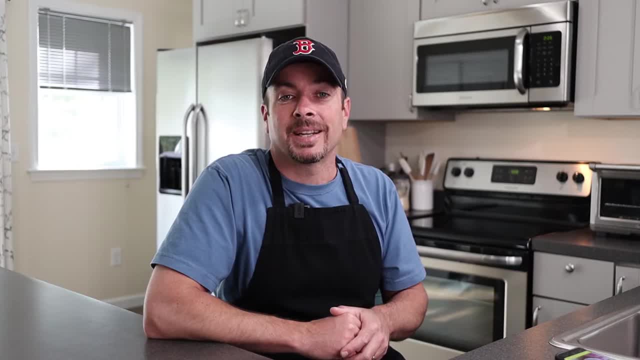 by cutting up your own whole chicken and you'll be shocked at how easy it is to break down a bird into the pieces of breast, chicken and beef. So I hope you enjoyed this video. I hope you enjoyed it And I'll see you in the next one. 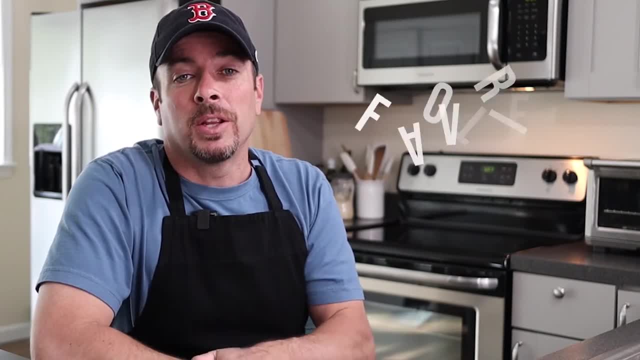 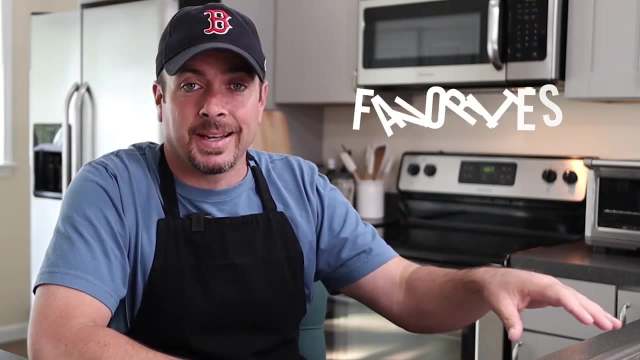 I really want to focus on the food that you like. So you might be watching my videos and be like that's not really the type of food that I like. But hey, jump in there and learn the techniques- the grilling, the sauteing and the braising- And then, if you don't quite have that recipe that you 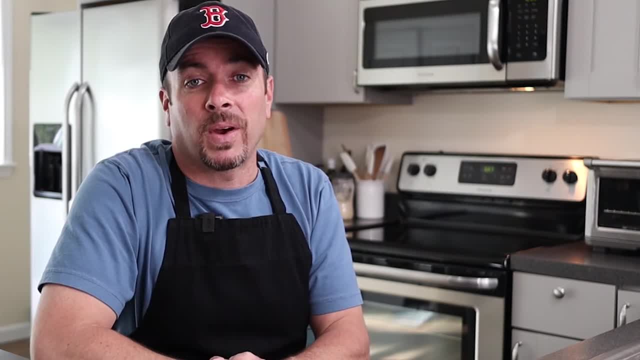 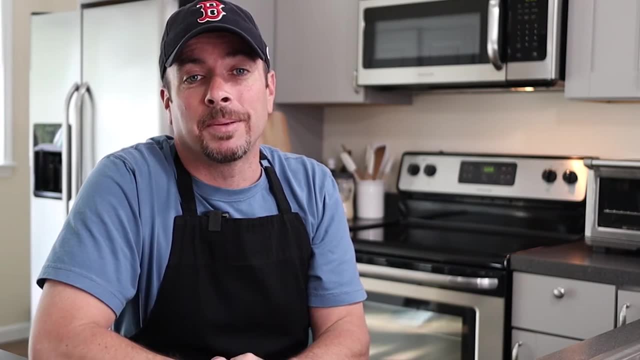 like that I make. then go ahead and find someone on YouTube to help you with that, or find a good recipe, Or let me know in the comments. Is there something you'd really like to see me cook or make? I'd love to hear from you. 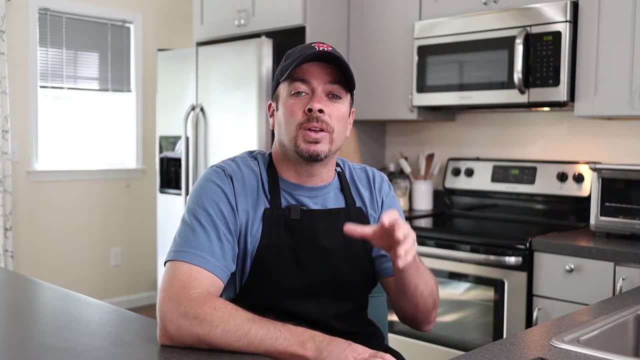 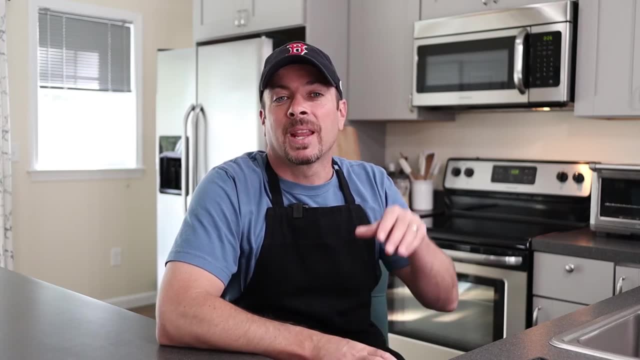 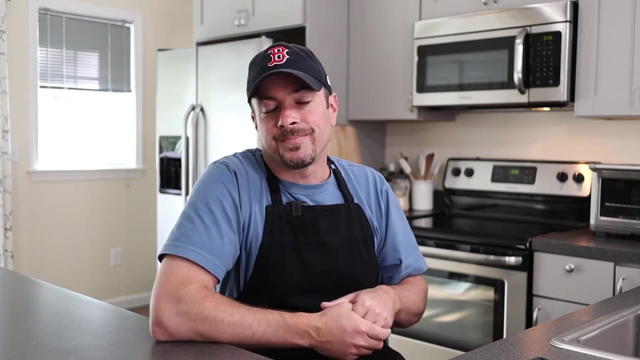 I'd love to hear what it is, But that's the thing I want to talk about. You really want to cook as a beginner, cook the things you really enjoy. So if you really like Italian food, start cooking Italian food. The techniques you're probably going to apply in most forms of cooking, whether it's 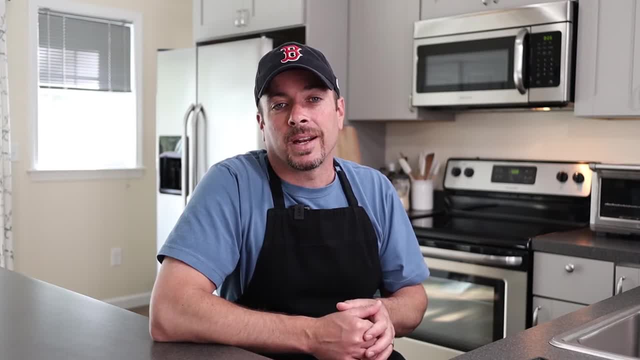 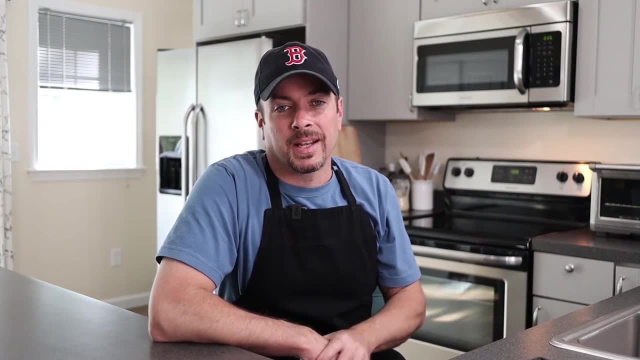 Italian or Mexican or Chinese food or you know. I don't even know if we have a certain type of food in America, But those techniques go across the board. So there's all kinds of things you can learn on my channel with skills and techniques, But that's the big thing. You want to cook the. 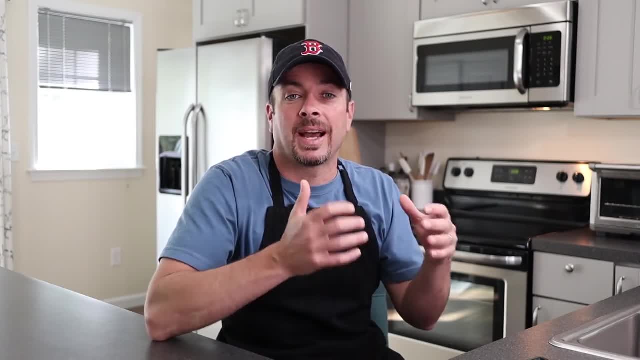 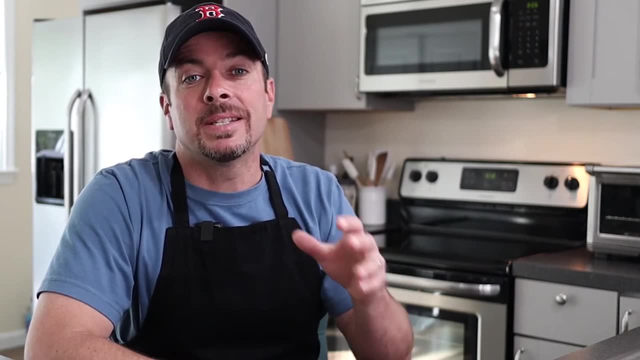 foods that you enjoy because you want to start to love to learn how to cook. Now I got one that's really big if you're a beginner cook and for all home cooks in general, is to season your food. Seasoning brings out the flavor in food. Some seasoning will bring out flavor, Some actually. 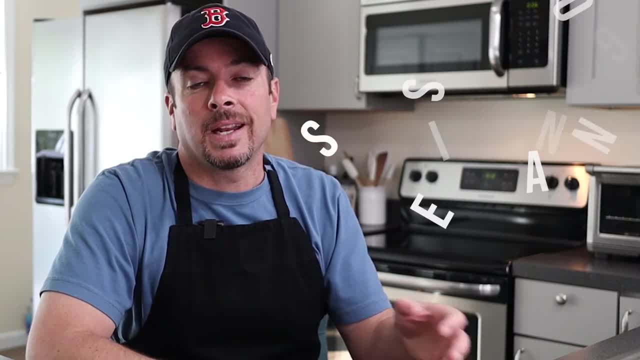 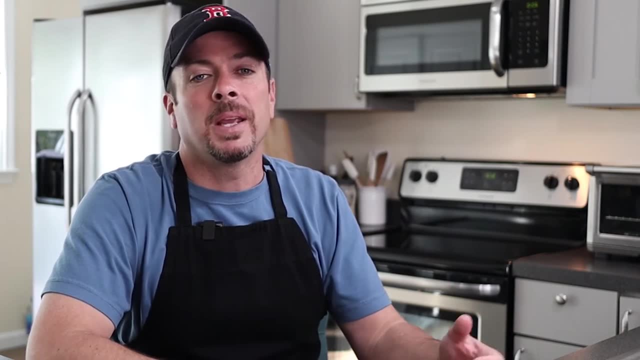 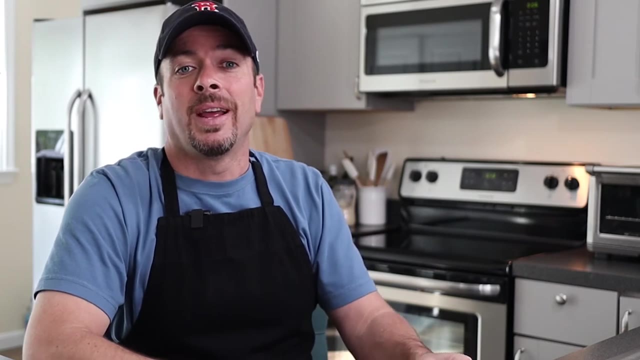 have its own flavor to it. But seasoning is so important- I hear it all the time. It's like my food just tastes so bland or the meal I created just tasted so bland. I'll tell you, probably 90% of the time it didn't have enough salt. So that's how important seasoning is. You really want to? 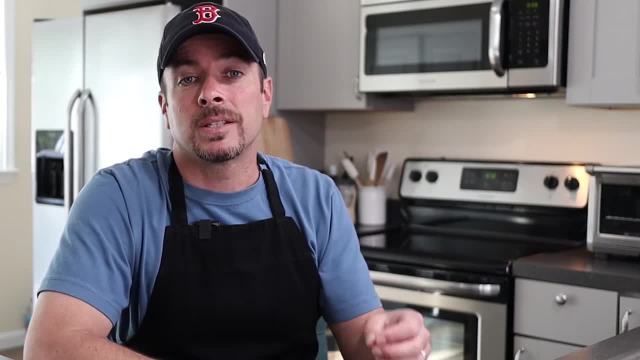 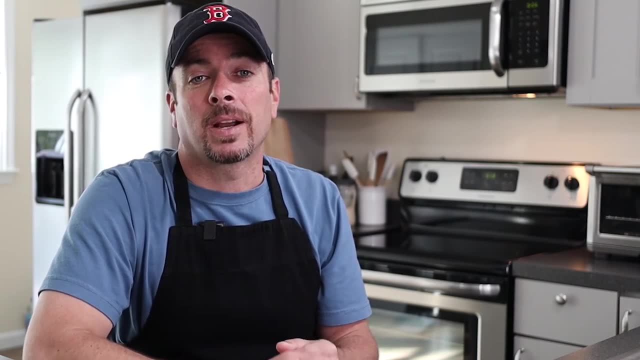 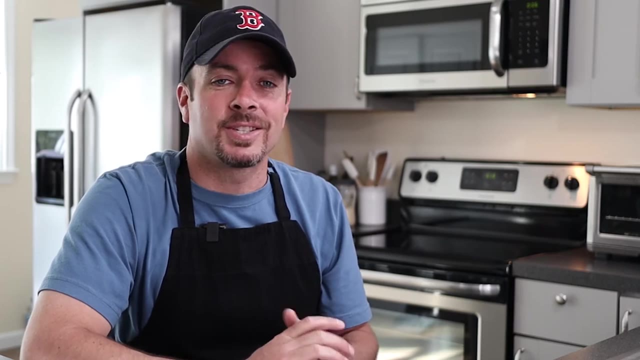 learn about seasoning your food with its salt. Salt enhances the flavor of your food, So it actually pulls out more flavor, And then there's things like pepper that add a complexity of taste or flavor to your food. Seasoning is so important, So that's something you really want to focus on as a beginner, And 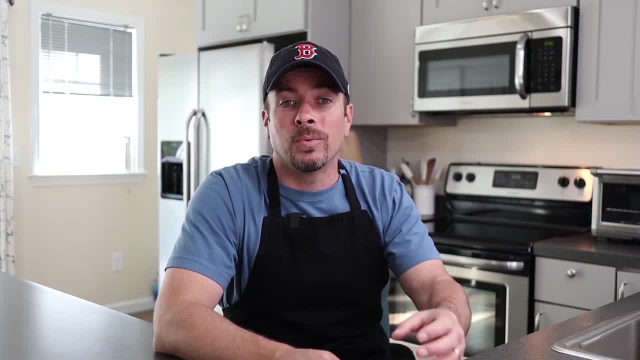 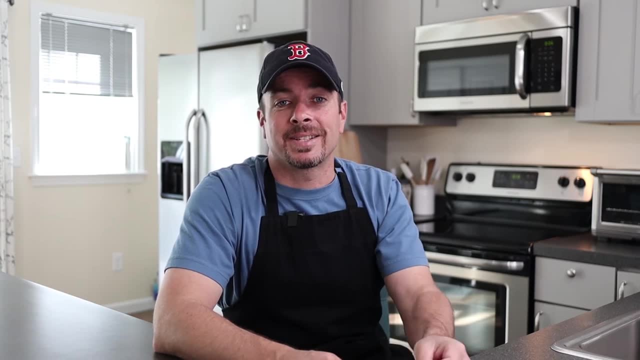 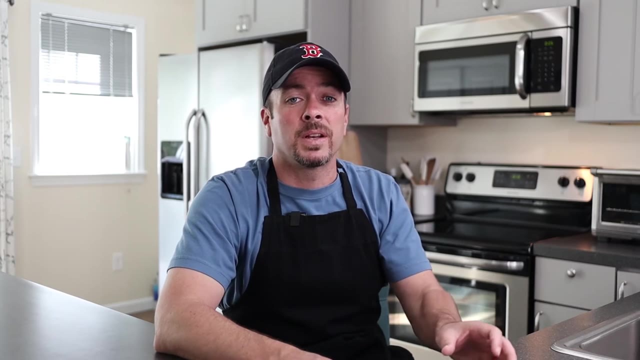 just do a little trick. Just take something you know, take a vine ripe tomato and eat it. Take two slices: Take one, eat it and then take the second one, put some salt on it and then eat it. Just do that simple test if you've never done it, and it'll blow your mind at the difference of 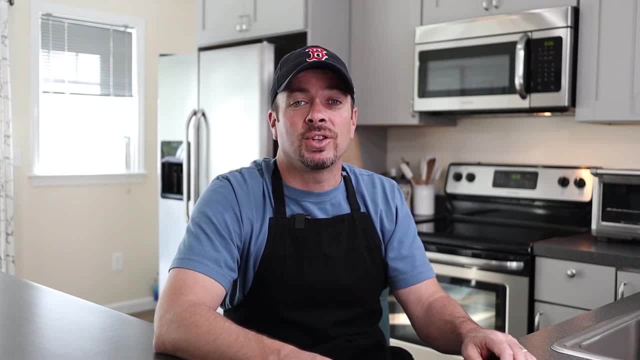 seasoning, And that's something I really focus on on my channel and on my blog. So all these things, too, are on my website, All the videos and recipes and how to's I do. I have a written form on my website you should really check out at homecookbasicscom, So this one is pretty important. 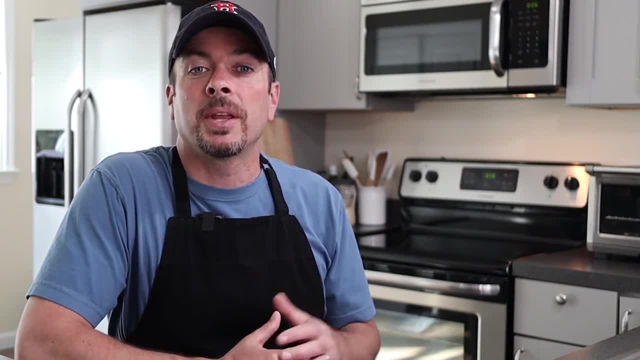 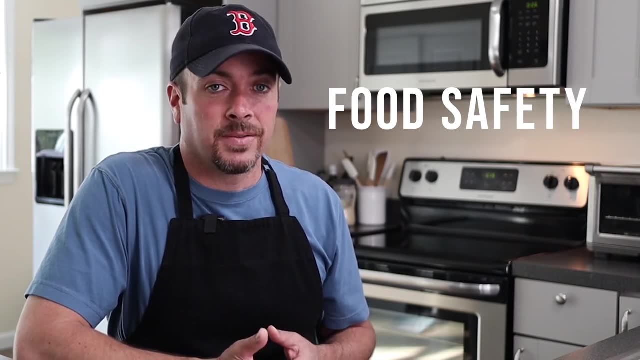 and probably you know it's not as fun, but food safety is really important. when you're learning how to cook As a beginner cook, you probably don't know all the differences and nuances of what raw chicken is and what temperature it has to be to be safe to protect yourself from salmonella. 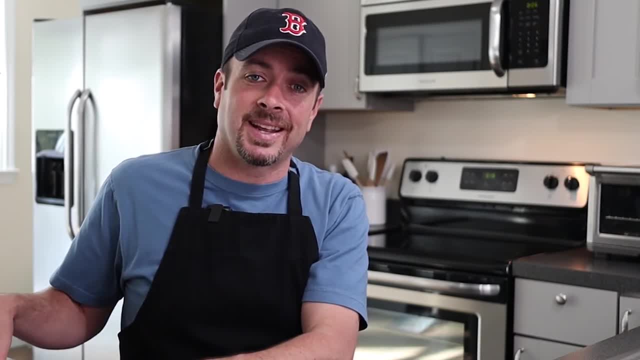 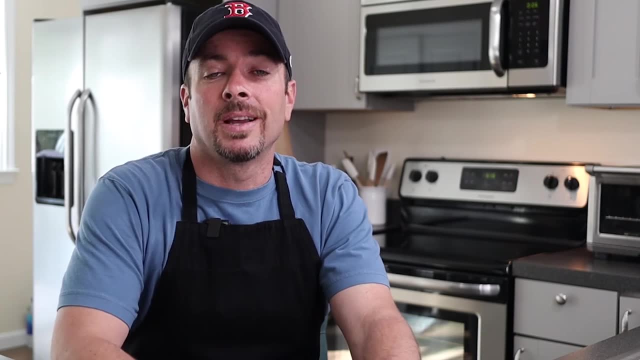 and things like that, And you know sanitation of cross contaminating, you cutting up the raw chicken and then maybe prepping some vegetables that are in a salad that you don't cook. So that's something you really want to focus on is learning a little bit of food safety and the sanitation a 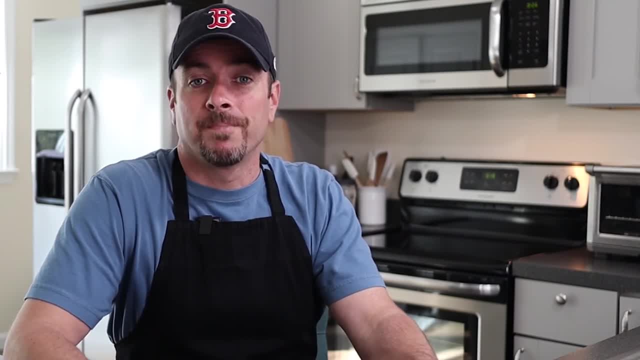 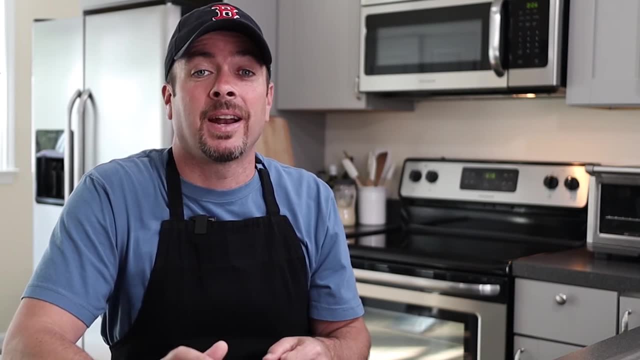 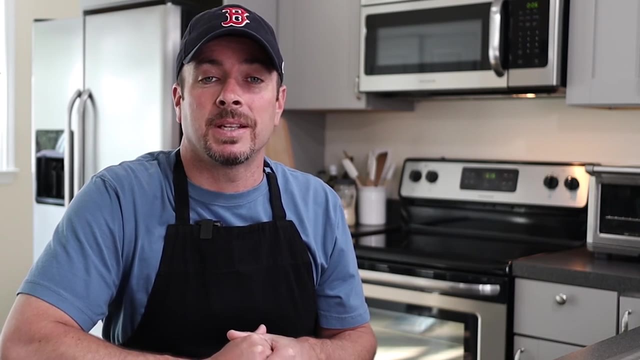 part of that- And you know, part of food safety too- is the temperature of the food that you don't want to serve raw food or food that's undercooked, that could be carrying harmful bacteria and stuff like that. 1 So that's. another important part of food safety is the temperatures of your food. 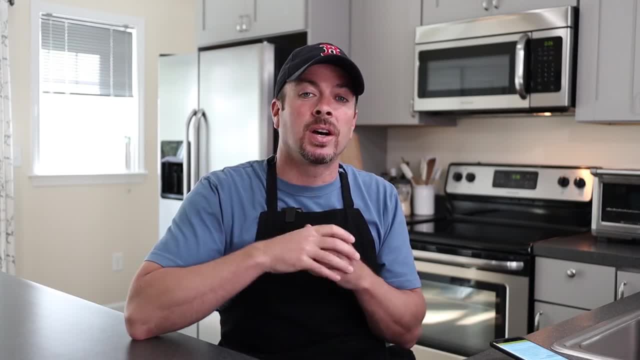 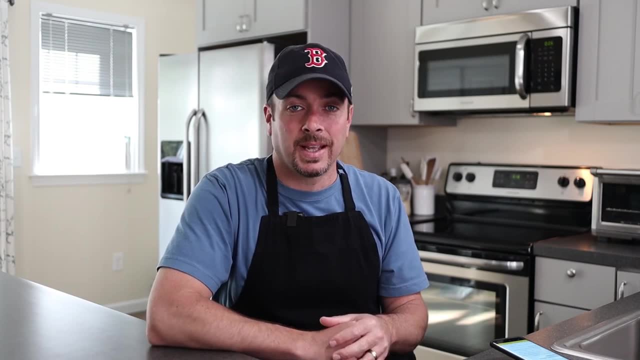 So, that said, I think that gives you a good idea, as a beginner cook- or you're just learning how to cook- of the things you need to know to just start out. I would focus on those things And, you know, one great resource is YouTube.